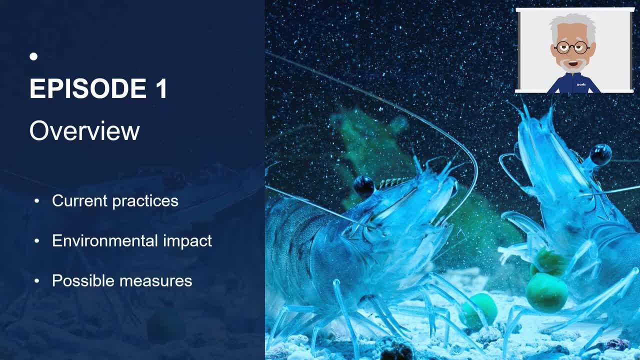 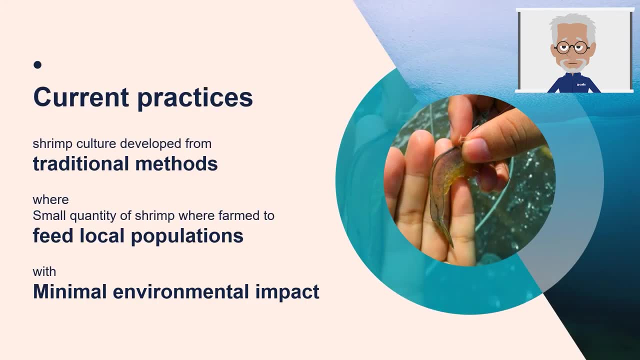 impact. Please note that much of what we will cover can also be applied to pond fish culture. Let's start by looking at current practices. Shrimp culture has developed from traditional methods Where small populations of shrimp can be used to grow fish, Where small populations of shrimp were cultivated to feed local populations with minimal environmental. 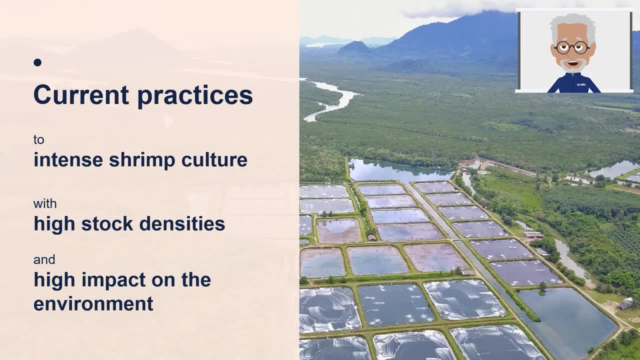 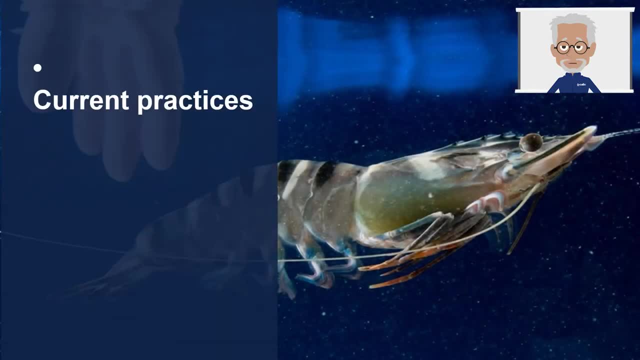 impact To a more intense culture with high stock densities and a much higher impact on the environment. There are a few common practices for shrimp culture: First, extensive. Second, intensive. Number three, clear water systems And number four, RAS, That's, recirculating aquaculture. 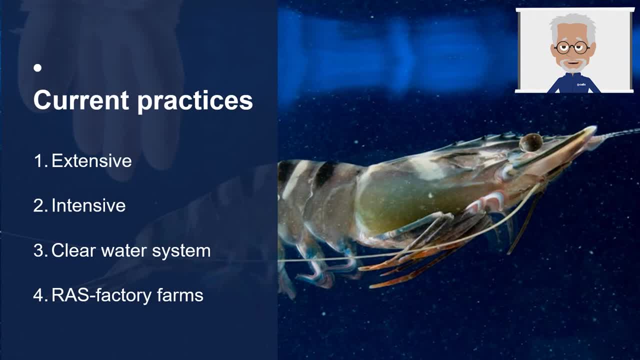 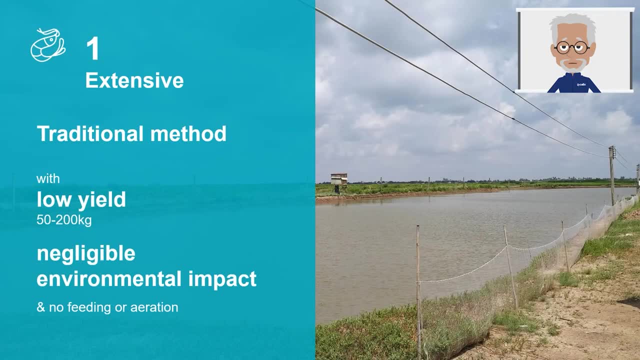 system, With the RAS system being a recycling system. it's only really used in China and the West. Extensive shrimp farming is often carried out in conjunction with fish culture. It's often used in small villages to feed local families or communities. This is the traditional. 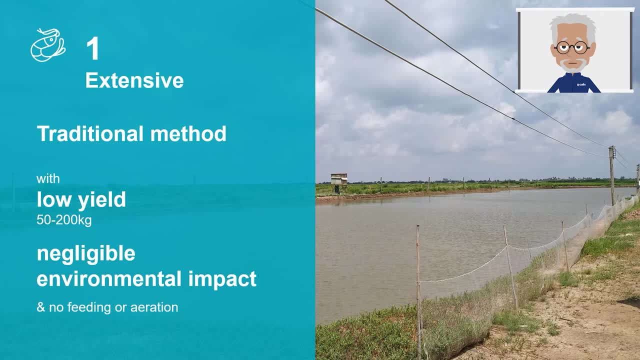 method used for shrimp culture. Yields are low, about 50 to 200 kilograms, and there's usually no feeding or aeration. The impact on the environment is usually quite negligible. Intensive shrimp farming is an extension of the traditional extensive culture, And it's 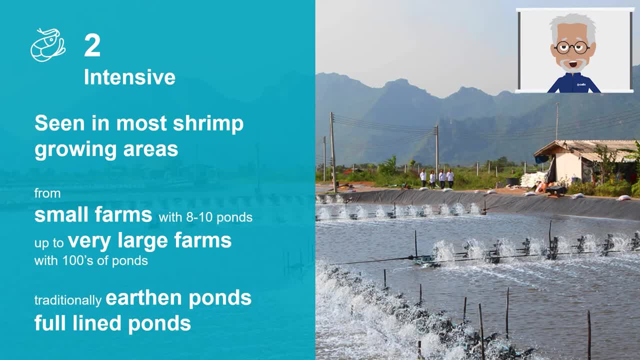 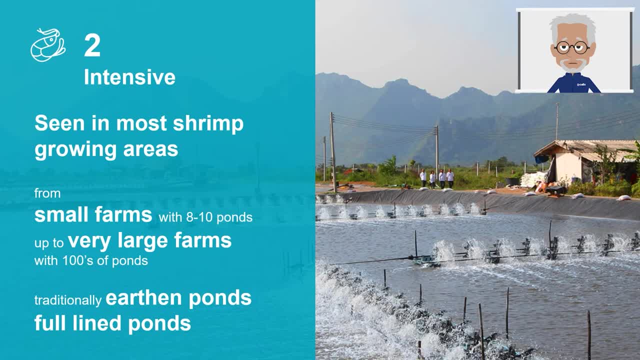 And it's a very common practice. And it's a very common practice. History is geared to producing shrimp at a larger, more commercial scale. History is geared to producing shrimp at a larger, more commercial scale. Many of these shrimp farms are traditional earthen ponds with aeration and chemical adjustments where 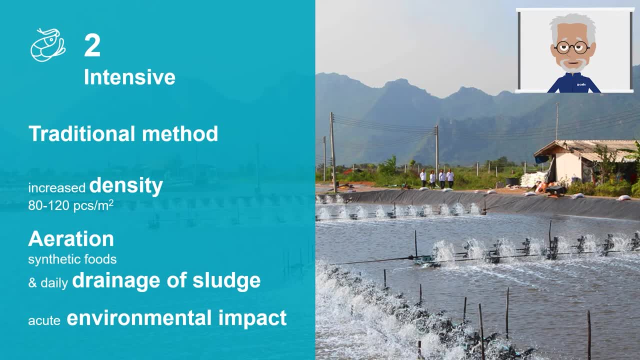 feeding is usually done with synthetic feed and drainage, And toxic sludge is commonly drained. This type of culture allows more intensive stocking: between 50 and 100 beasts per square metre. As demand for shrimp increased in recent years, many of these farms have also adapted lined 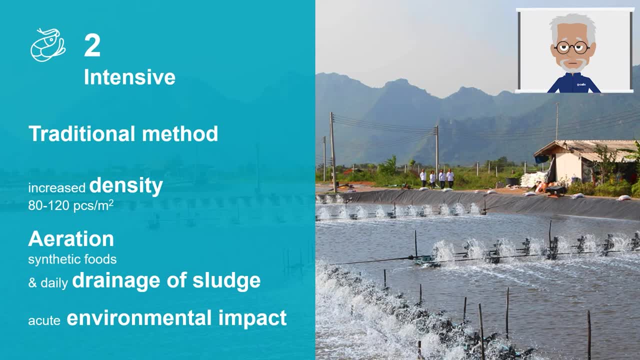 ponds enabled them to increase their stock densities up to 150 to 200 ppm. As stock density increases, the need for drainage of toxic sludge and water exchange increases. This is precisely what, for many farms, poses a major operational issue and thus an environmental. 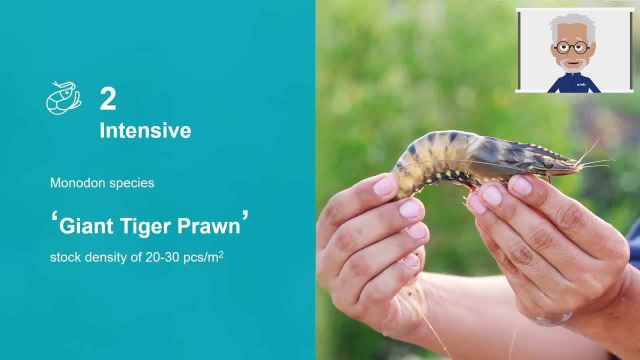 challenge. These intensive shrimp farms have traditionally been farming monodon, commonly known as the giant tiger prawn in Asia, with stock densities of 20 to 30 ppm. However, in recent years, another species known as the Pacific white shrimp from South 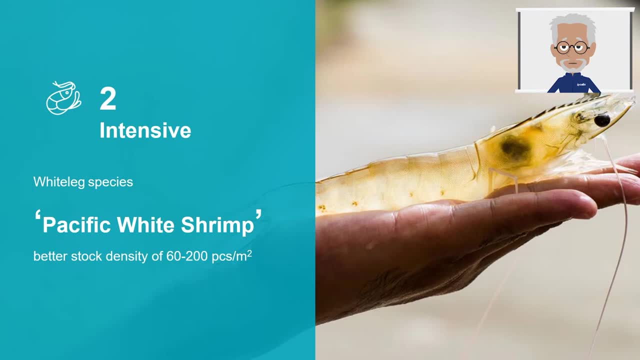 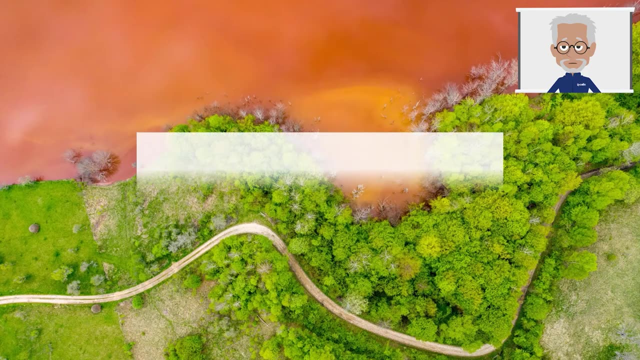 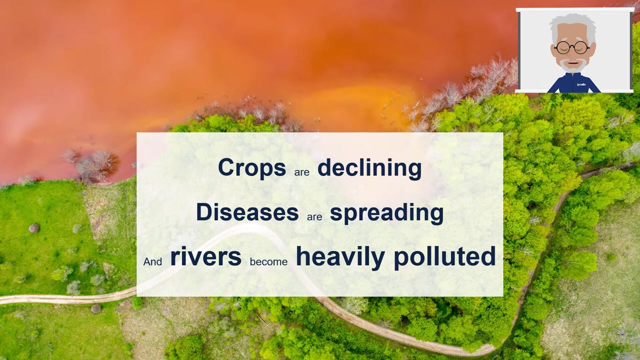 America has also been introduced, with many farmers making the switch as this species grows faster, with great stock density of 60 to 200 ppm. We hear the same story from many of our farmers across Asia. The first years of culture produced consistent and profitable crops with little instance. 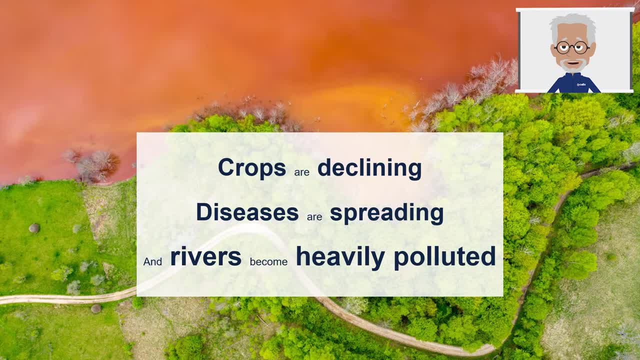 of disease. However, in recent years, crops have started to decline and instances of disease appeared to be more widespread. The river systems and coastlines in these intense culture areas are often heavily polluted with toxic discharge from farms. We believe this is one of the primary causes of reduction in yield and the increase in. 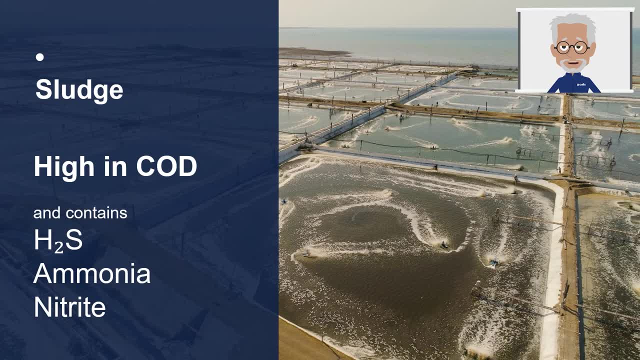 diseases. So why is sludge so bad for the waterways? Well, it's high in COD, that's chemical oxygen demand. This means it affects oxygen. It contains toxins like hydrogen sulphide, known as H2S, ammonia and nitrite, and they're. 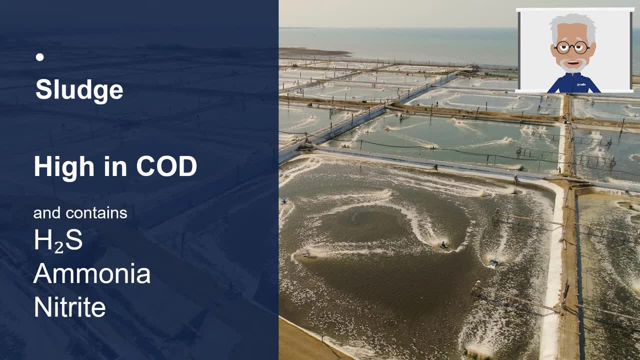 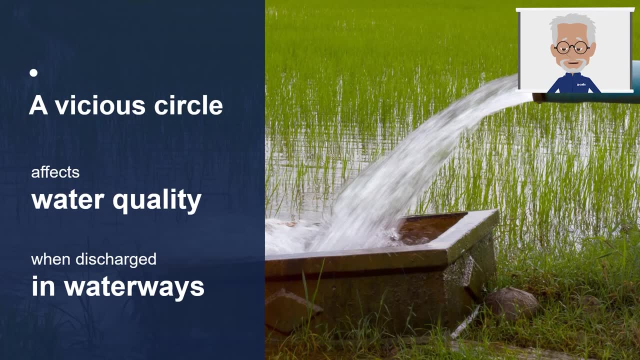 all really bad for shrimp culture and an ideal breeding ground for viruses and diseases. When this nasty sludge is discharged into the waterways, it can affect the quality of the water which the farmer needs for his day-to-day operations. So this then becomes a vicious circle and it progressively gets worse and worse at the 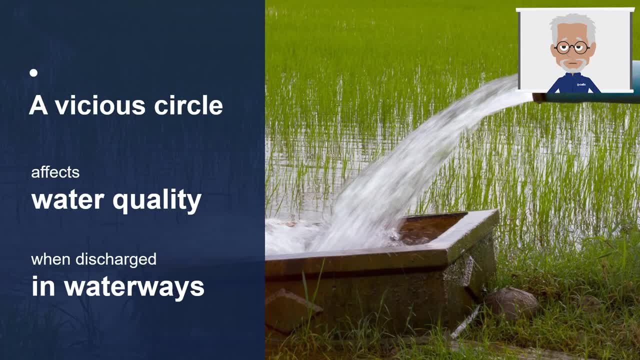 lower end of the system. In fact, as waste from farms upstream increases, so does the water. In fact, as waste from farms upstream increases, so does the water. When the water stream is discharged, it affects the water quality but also the bottom of the 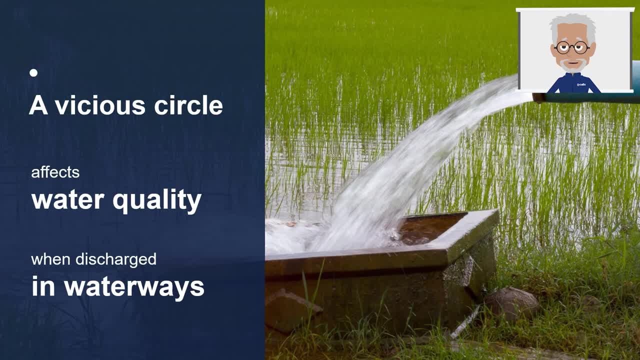 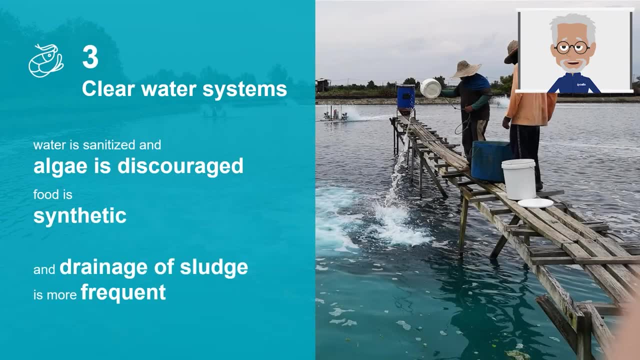 waterway. It's like discharging raw sewerage into your system, which means you're introducing unwanted disease and pollutants in your farm. Intensive shrimp farming was based on a green water system, where farmers cultured beneficial algae that could supplement synthetic feed, particularly in the early stages of the culture. 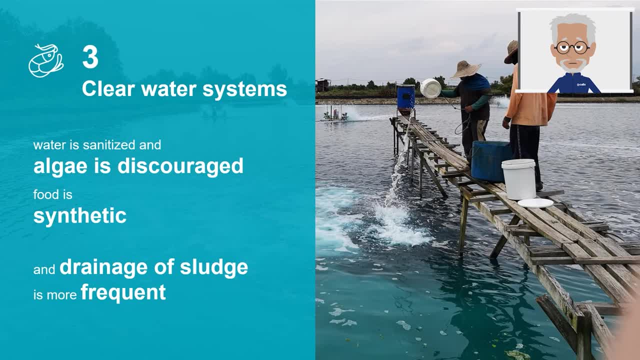 But in recent years we've seen an increase in the introduction of clear water systems. Feed water is treated and sanitized in a reservoir and algae are destroyed or discouraged in this system, And this makes clear water totally dependent on synthetic feed with drainage of toxic. 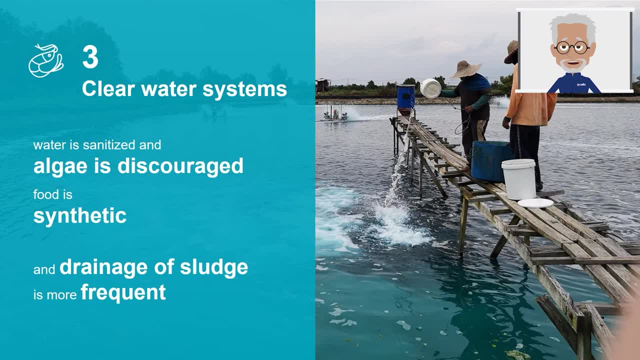 sludge becoming a lot more needed and frequent. This method recommends that all sludge is treated in a further pond system. This clear water system also increases the cost of culture dramatically. It impacts the cost of chemicals needed and reduces the available cultivation area on. 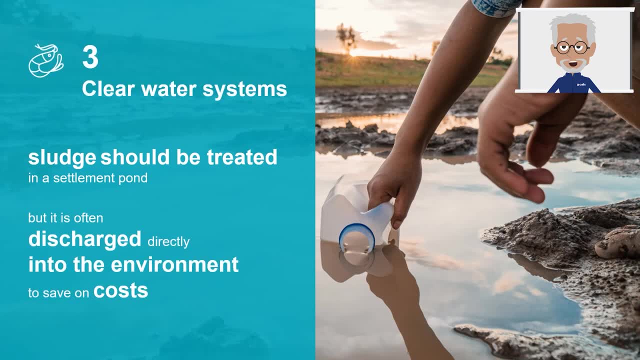 a farm. In fact, this method also reduces the cost of chemicals needed and reduces the available cultivation area on a farm. Even clear water systems do not always treat the sludge adequately and it's often discharged directly into the environment to reduce costs. 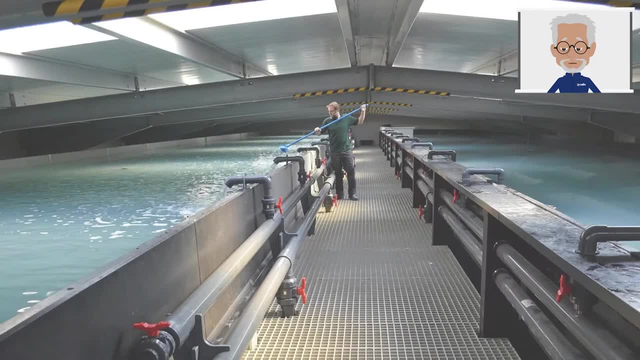 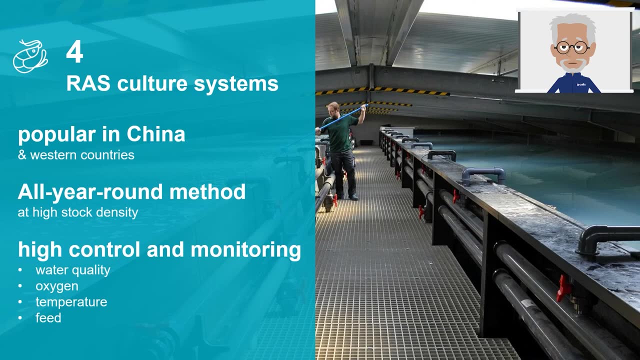 This pollution poses a critical risk to the environment. Let's now have a look at recirculating aquaculture systems- RAS. These are gaining great popularity in China and the West. In this culture method, shrimp and other species can be farmed all year round at high stock. 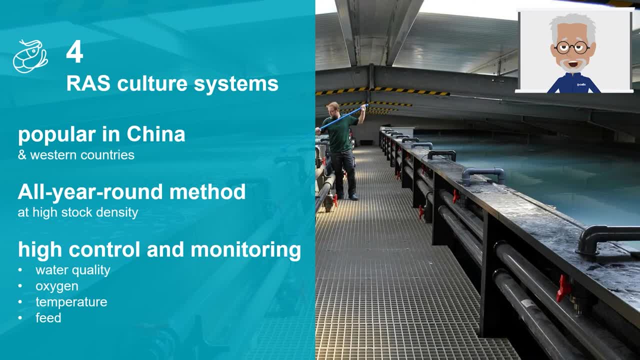 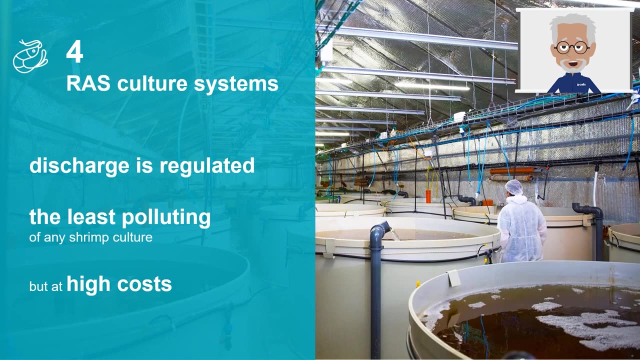 densities. Recirculating aquaculture systems are usually highly regulated by the farmer here He himself, with strict attention being paid to water quality. Water temperature is controlled, along with pH, alkalinity, ammonia and nitrite. Discharge is often regulated by local authorities. 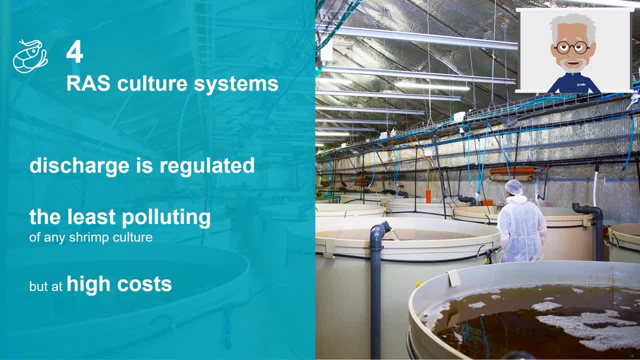 All this makes RAS probably the least polluting of the shrimp culture's practice today. The downside is the high cost of infrastructure, the stringent environmental control and the cost of waste treatment. Of the many systems used commercially, most impact on the environment and less strict. 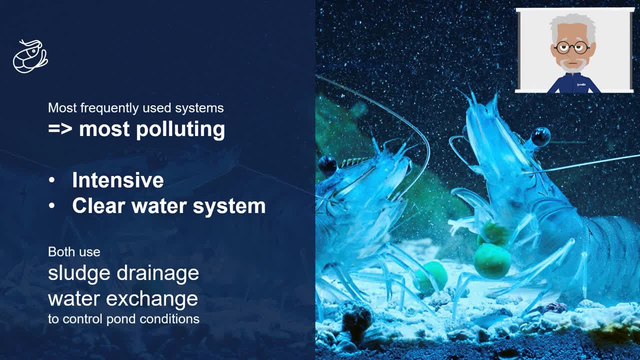 controls are applied. Of course, it's the most frequently used systems that pose the highest potential risk for environmental impact, and they are intensive farming and clear water farming. Both of these methods require frequent sludge drainage and water exchange and, as we've 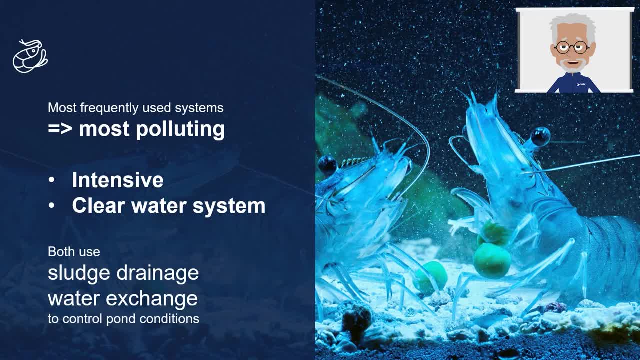 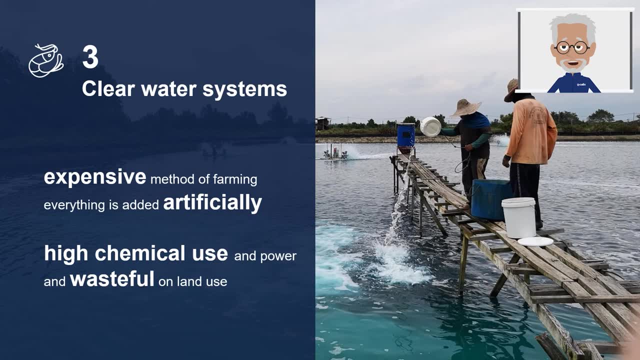 seen previously. this can really impact the waterways and the farm's productivity. Clear water or CP system is a system where water is sterilized and suspended. solids and nutrients are removed from the grow out area. This means that natural nutrients and minerals are removed. 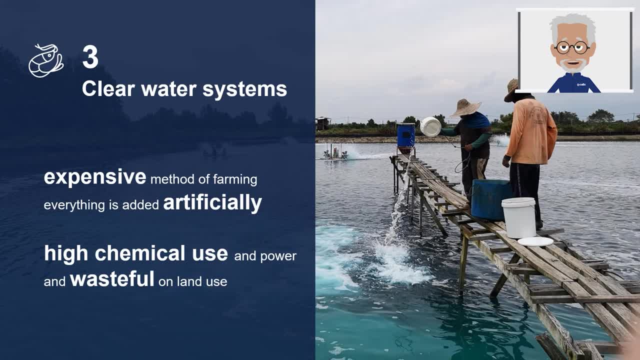 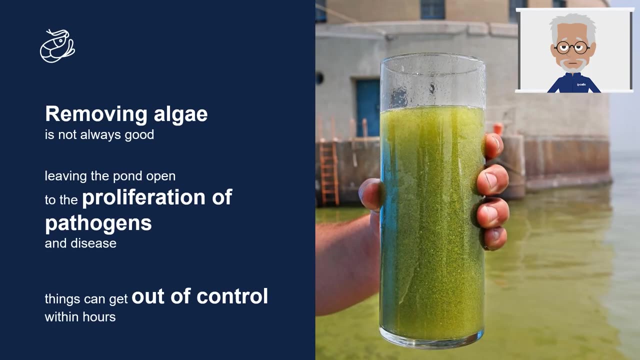 It's an expensive method of farming, as everything needed for the pond to grow must be added by artificial means. This is why it's extremely expensive in chemical use power and is also wasteful on land use. The idea is to reduce the proliferation of disease, but unfortunately nature abhors. 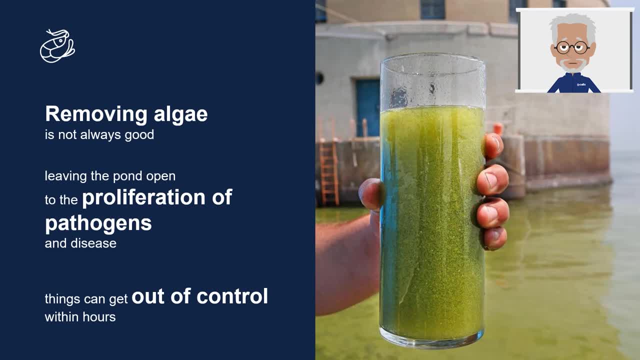 a vacuum which is in fact created when removing beneficial algae. So if the farmer doesn't sanitize correctly or exercise properly, then the plant will have to exercise correct biological protocols such as stopping birds, insects, lizards, monkeys gaining access to the ponds or wind and flood waters entering the farm. then there's a 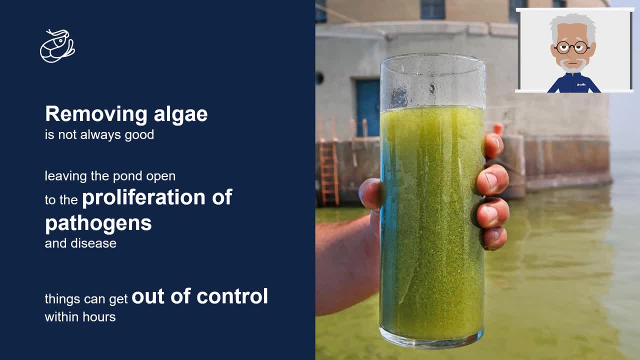 high chance that pathogens, virus or fungi are introduced, As there is no dominant species of algae in the pond and free chlorine can't exist in conjunction with the culture. this leaves the ponds open for the proliferation of disease, And it only takes four to eight hours for things to get out of control. 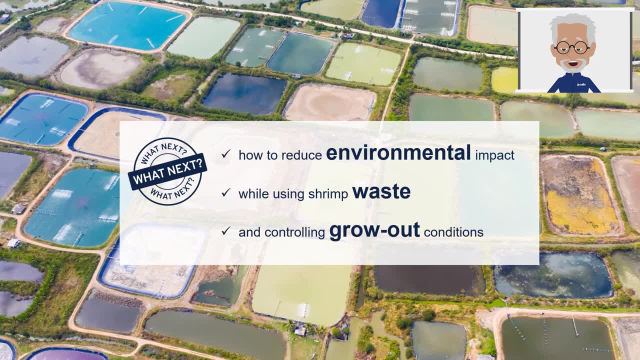 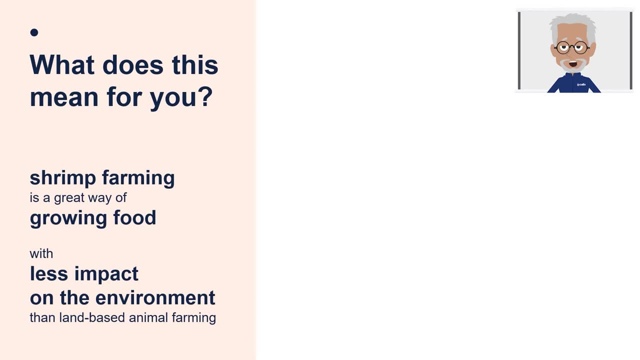 In future episodes of this series, we'll investigate how to reduce environmental impact while using shrimp waste and controlling grow-out conditions. So what does this all mean, and what does it mean for you? Aquaculture is a relatively new industry with a bright future, but in some cases, it still. 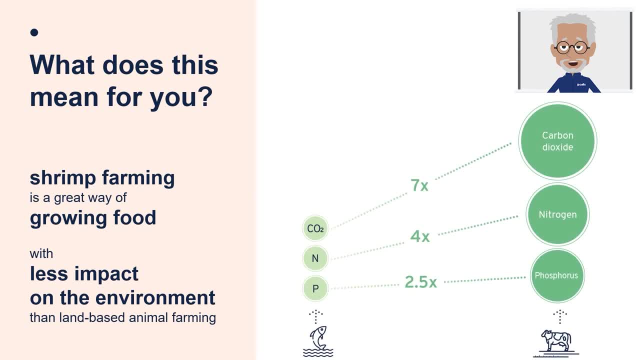 has a long way to go. Theoretically, aquaculture and shrimp farming can and should be a more efficient way of growing food with less environmental impact compared to land-based animal agriculture. As scientists' understanding of these impacts and risks increases, regulators and farm 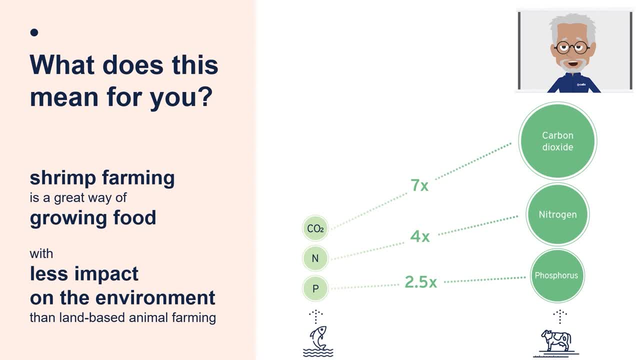 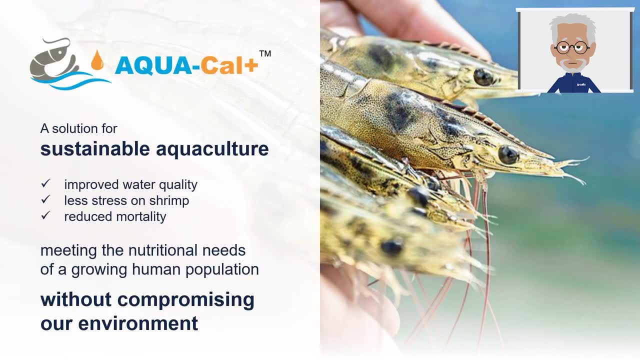 managers can start implementing strategies to protect their farms and the environment they depend on, With passion and a purpose of solving global challenges. Calix has developed AquaCal+, a water conditioner that safely addresses disease, improves productivity to sustainably meet the nutritional needs of a growing global population. 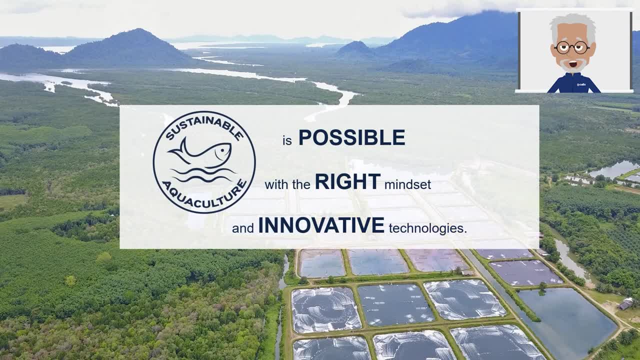 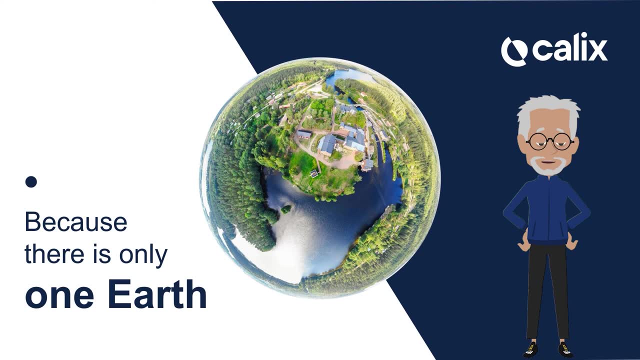 Sustainable aquaculture is possible. It's possible with the right mindset and innovative technologies Because, as we like to say here at Calix, there's only one Earth and it's already ours. Mars is for quitters. Thanks for your attention. 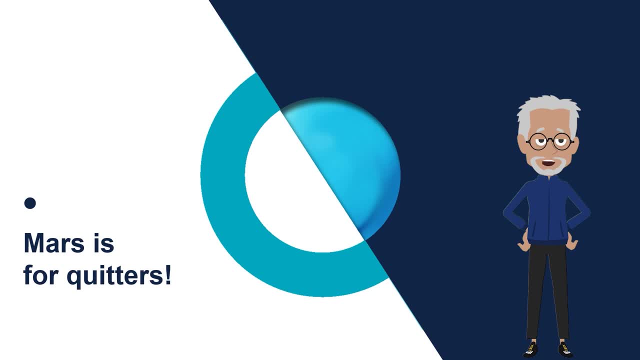 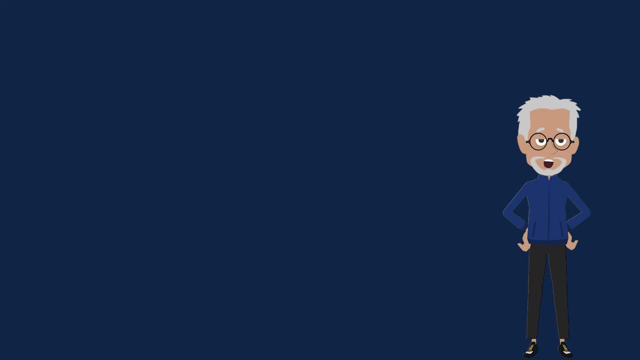 We hope you found this video interesting and I hope you'll join me again for the next episode of this series on sustainable aquaculture. To find out more about us or about AquaCal+, visit our website at wwwcalixglobal- wwwcalixglobalcom.